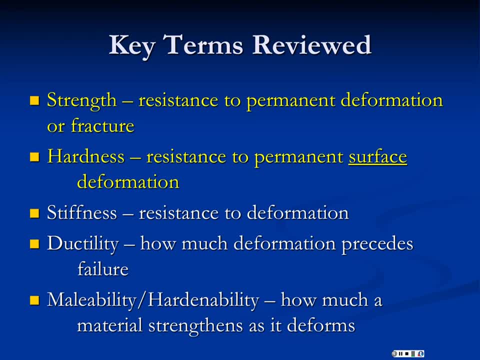 Hardness is related and it's also permanent deformation, but it's surface deformation. Other terms that we've alluded to- and we want to be sure we keep straight- stiffness is an overall resistance to deformation. You may think in practical terms of the difference. 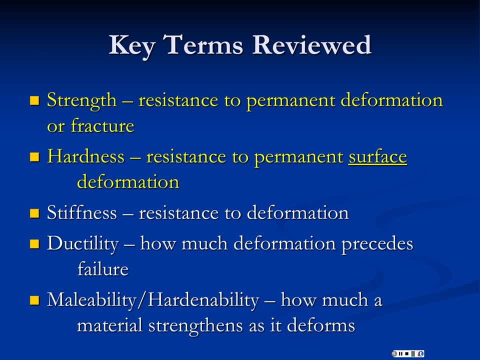 between the stiffness of a piece of foam and a piece of wood, One makes a much more comfortable seat than the other. It's because foam gives, and so that resistance to deformation we refer to as stiffness. We're going to have engineering terms that apply to all of these Ductility, as we talked about. 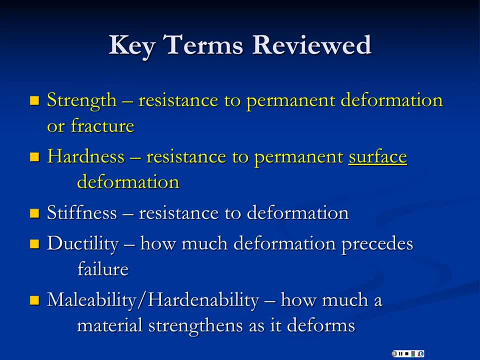 last class is how much deformation precedes failure, And the malleability is one way to talk about hardenability, and that is how much a material strengthens, that is, how much it becomes more difficult for it to deform as it deforms, as continued deformation occurs. 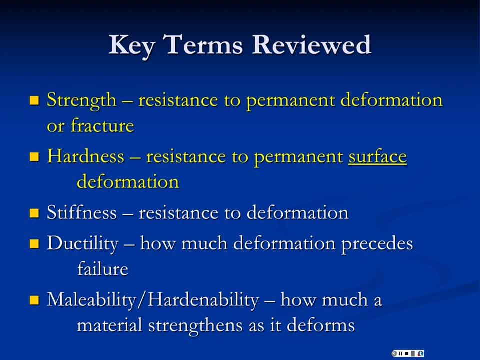 So we will be throwing these terms out again. So we're going to look at the strength of deformation and we're going to look at how much deformation precedes failure. So we're going to do that again today and in most of our following classes for the next couple. 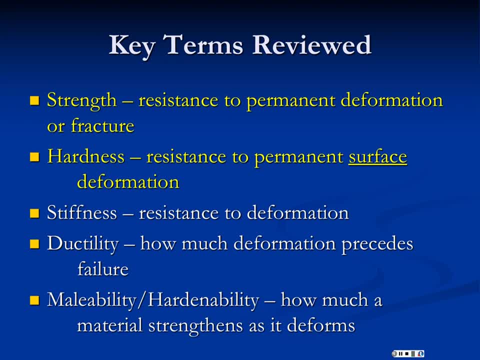 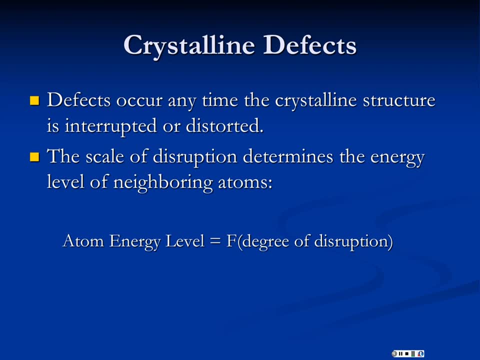 months. So you need to be very clear on those. All right. so crystalline defects: What is a defect? And defects are not necessarily bad things. We're going to have defects that we intentionally introduce into crystals And simply a defect occurs if a crystal structure is interrupted or distorted, It is not its 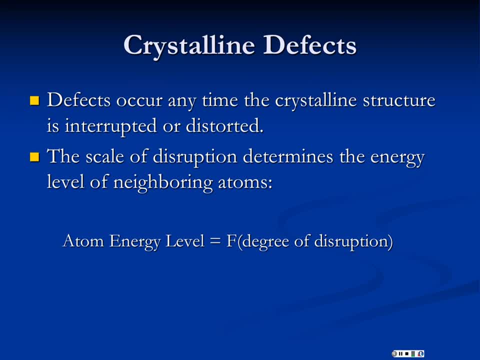 ideal structure And the scale of disruption is going to determine the energy level of around that disruption. So basically you can think of the energy level of atoms in a crystal is a function of how much they are disrupted from the minimum energy state of a perfect crystal. 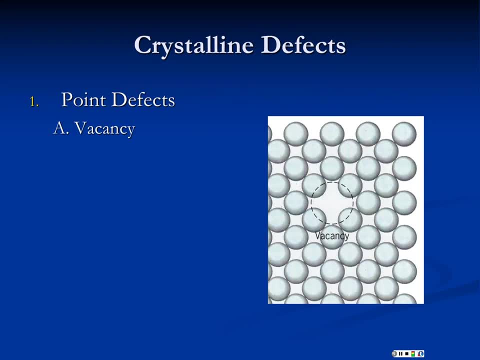 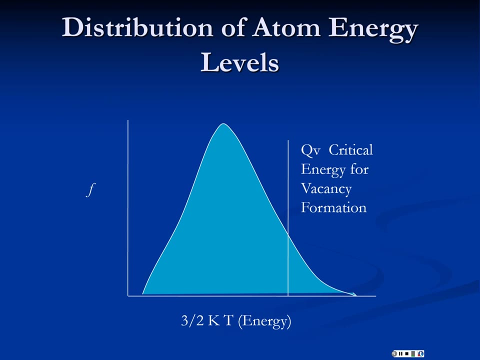 The greater the disruption, the greater the energy. So the first of these defects is simply a missing atom. It's called a vacancy And very simple, And this is caused by thermal excitation. So if we go back to week one, we talked about what temperature is And that temperature is. 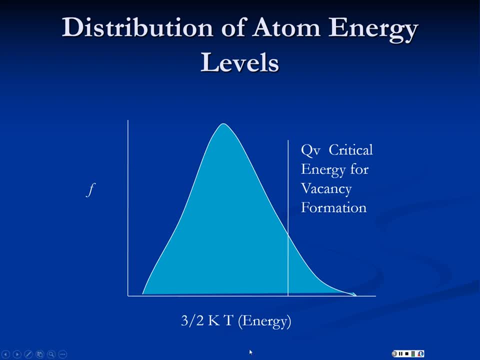 a measure of the energy of particles. You remember we had that the kinetic energy of atoms or molecules is equal to three halves kT, where k is Boltzmann's constant and T is the temperature in the absolute scale. So temperature is a linear predictor or is a linear measure? 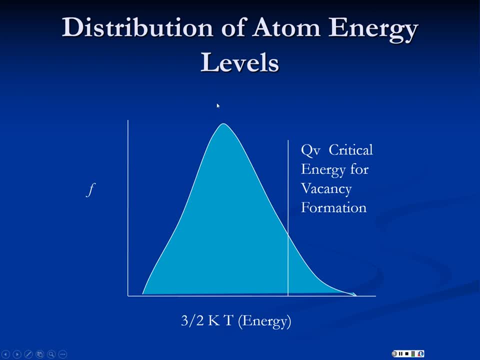 essentially of the kinetic energy of the particles At a given temperature. so this is my mean remember we have a distribution of temperatures actually present. Some molecules are hotter, some are colder. Now a vacancy requires that elevated energy be present. The neighboring 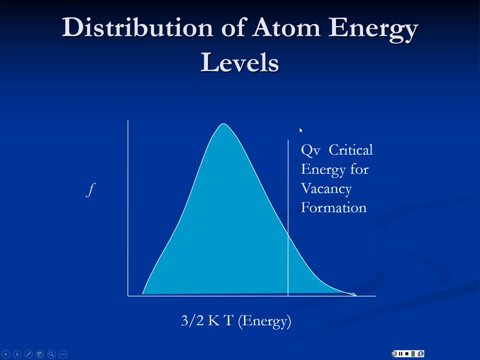 atoms are missing a neighbor, so they have higher energy, And so that energy level is called QV. It's the threshold energy required to form a vacancy, And what you recognize here is that if this is my QV and this is our nominal temperature, I'm going to have a few vacancies. 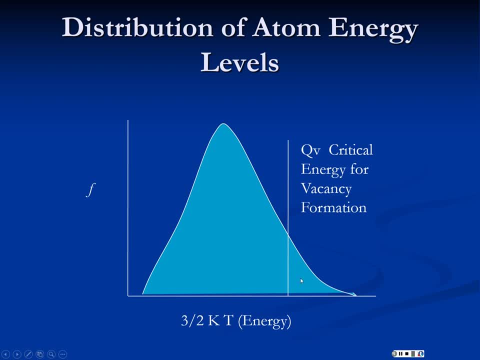 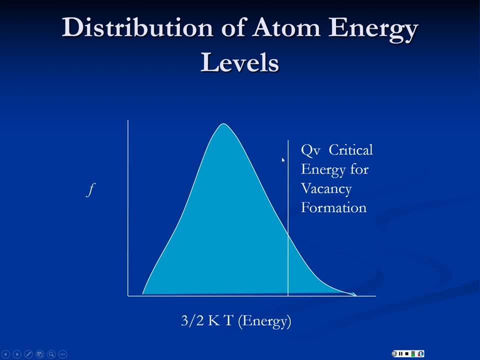 as we raise the temperature, more and more of this distribution will be higher than this QV energy level And we'll get more and more vacancies. But it's not a simple linear function. So it turns out that the number of vacancies is an exponential function of temperature. 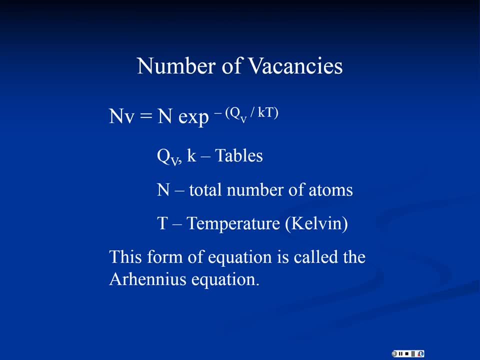 And this is a form you're going to see many times in this class- where we have what we call an equation type And the name of this equation type is an Arrhenius equation- It's named for a Swiss scientist who first proposed it. The basic structure is: we have an exponential 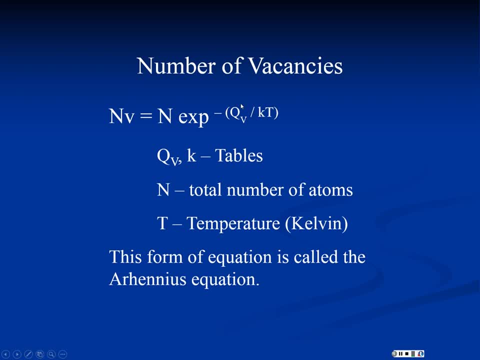 function where there's a Q in the numerator- and this is the energy barrier that has to be jumped- There's always a constant, and it may be K, which is Boltzmann's constant, and it also may be R, the ideal gas constant, depending on the problem, And then T is always. 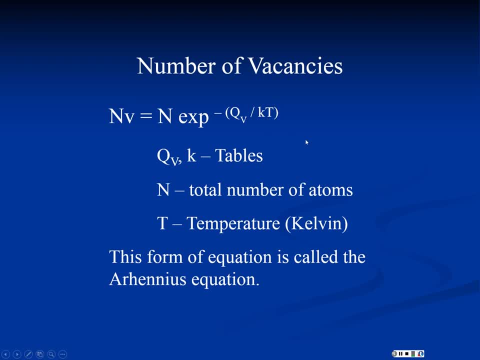 in the denominator as well, And that's your temperature, And that's your temperature in Kelvin. And so just a reminder: we already told you that if you are doing temperature in this class, use Kelvin always, and you'll never be wrong. 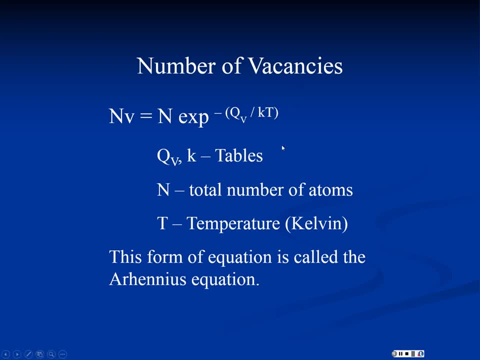 If you do this problem in Celsius, you will not get correct answers. So N is simply the total number of atoms present, and V is the number of vacancies. You'll often see this written as NV over N, That is the fraction of atomic sites that are vacancies, And so then you get NV over N is. 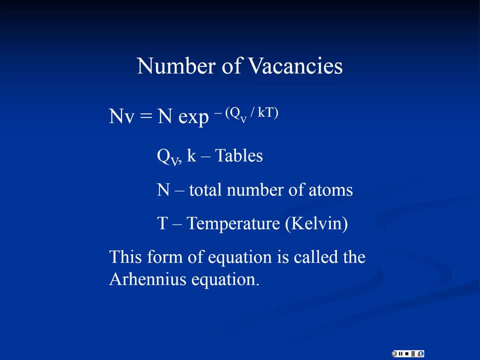 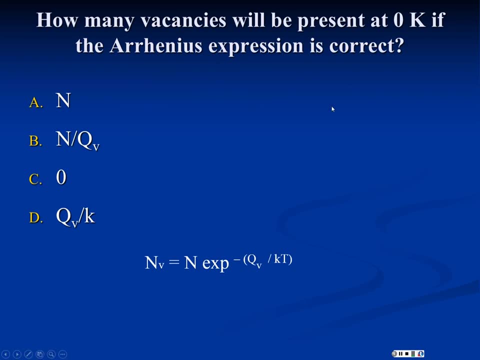 equal to this exponential term. Now it has a very special form here, So it poses a question to you: How many vacancies will be present at zero Kelvin, if this expression is correct? So pause the audio at this point and take a moment and see if you can figure out what the answer is. All right, Let's do. 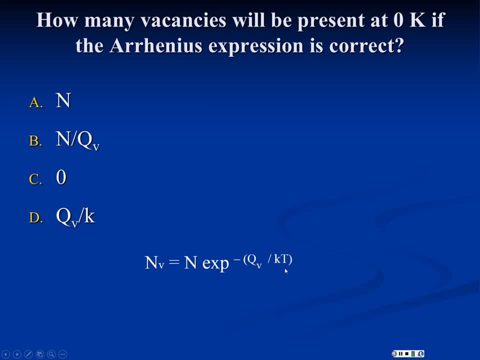 the analysis. If you plug in zero T here, this is a number divided by zero, which is mathematically obviously undefined. but we would say that's infinity, The limit. as temperature you can't have absolute zero, but as you approach absolute zero, this value approaches infinity. 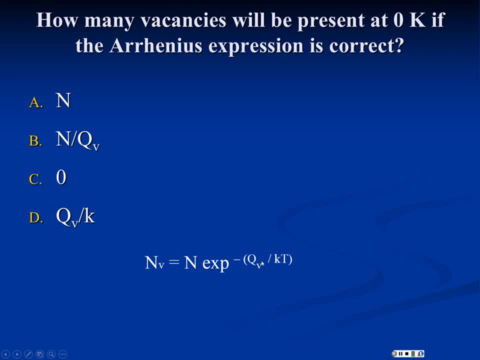 So if I'm taking E to the negative infinity, well E to the infinity is infinity, but this is a negative, so it's a reciprocal. So 1 over E to the infinity, so 1 over infinity is zero. That is, this doesn't have any meaning at zero, Kelvin. 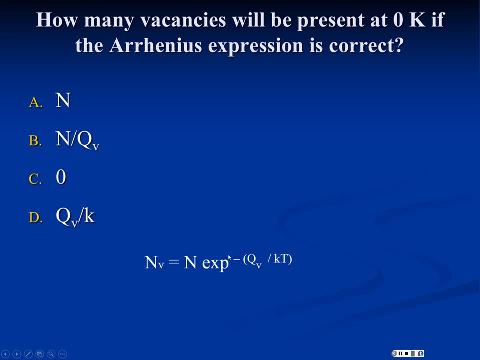 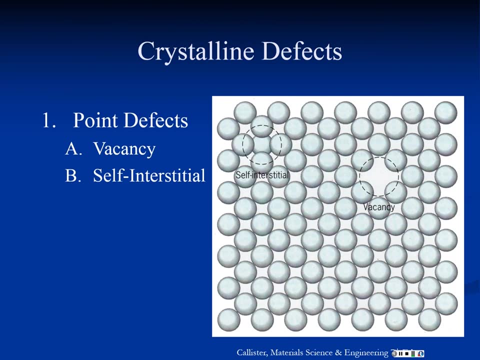 but we can't get to zero Kelvin. But as we approach zero Kelvin the number of vacancies actually goes to zero. So you will have a perfect crystal only at very low temperature, All right. second kind of point: defect is a self-interstitial 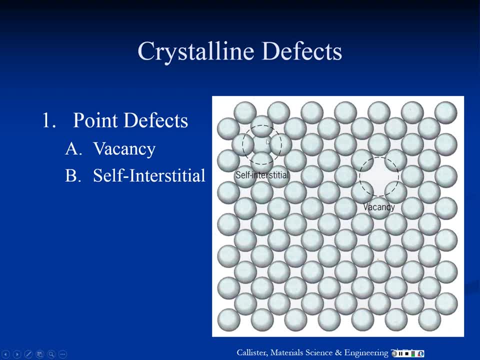 It's just an extra atom jammed in here. Obviously, this takes a lot more energy than a vacancy- These are much less common than vacancies- and a self-interstitial plus a vacancy and you get nothing. They annihilate each other. 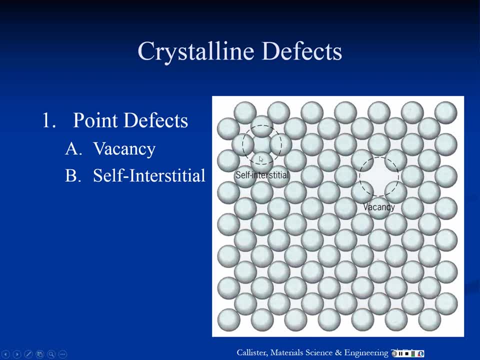 So these are not particularly common. They tend to appear and disappear relatively quick And they're going to be important in transitional forms, particularly in some weird ceramic structures, but we're not going to do much with them in this class, All right? so at this point let's step back and ask: 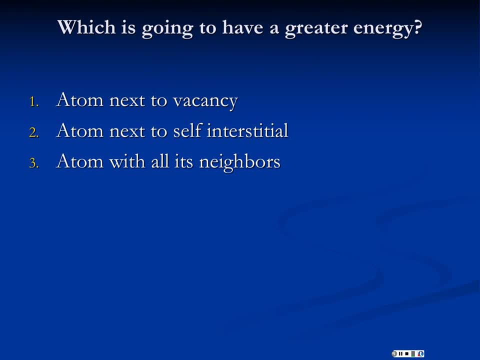 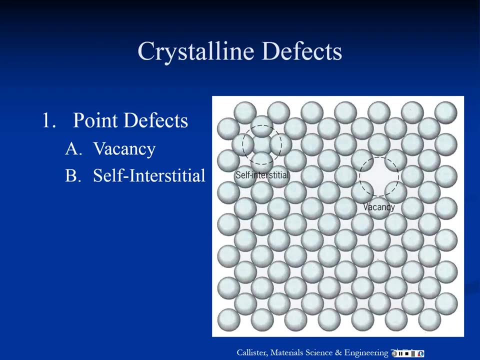 which atom is going to have a greater energy? One next to a vacancy, one next to a self-interstitial, or an atom that's got all of its neighbors? When you think about this, there's no. Let me just be logical here. 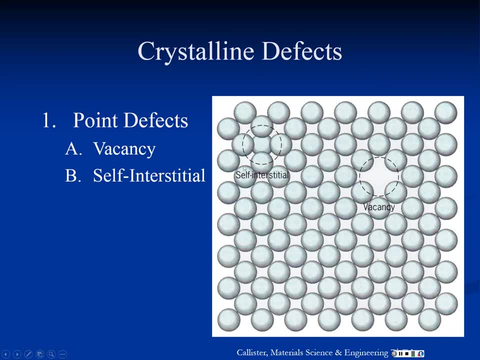 Is this an atom around this vacancy, an atom around the self-interstitial, or one of these atoms out here that's got a perfect neighborhood And most likely you're self-interstitial because there's a serious interference going on here, So it's going to have very, very high energy. 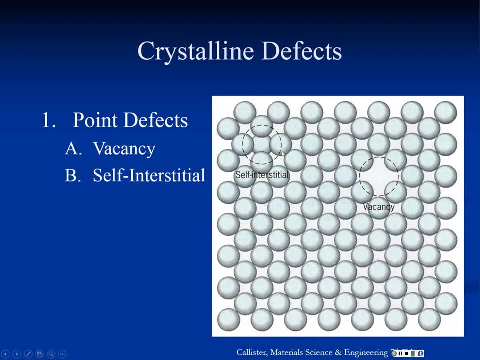 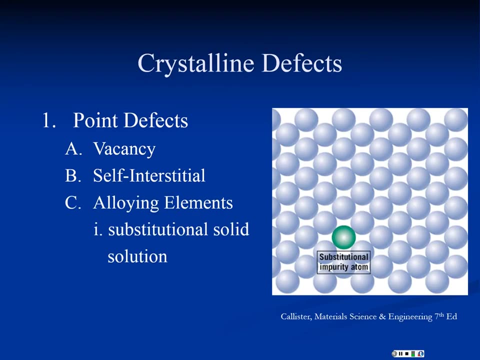 which, as we're going to learn later, is going to give these atoms a tendency to diffuse or leave this location, And so it's another way self-interstitials disappear is we'll get a succession of atomic movements that fill a vacancy. Okay, now we get to the really interesting point: defects. 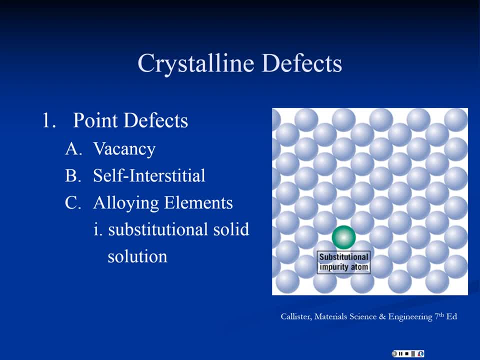 The first of these is a substitutional atom And understand from the perspective of this crystal, an atom of a different element that is similar but not identical. even though the crystal structure does not appear to be disrupted, it is not a perfect replacement. 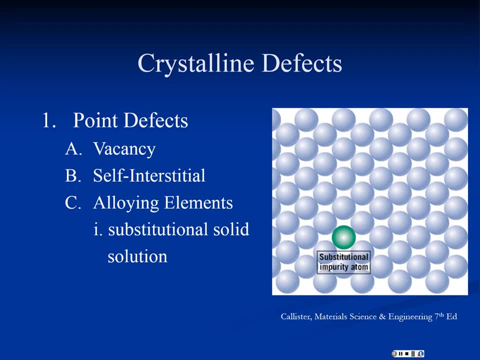 And so it will raise the energy level of all of the surrounding atoms. From the perspective of the crystal, it is a defect, And we're going to do this intentionally a lot, because it's a way to alter the properties of the material. So the first of these is a substitutional impurity atom. 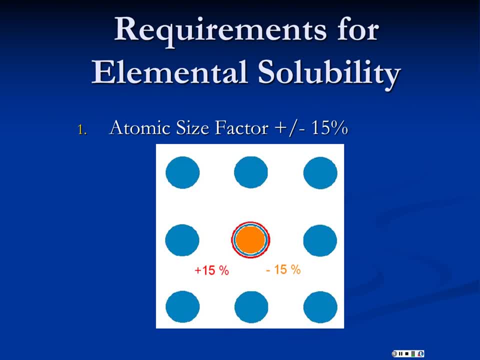 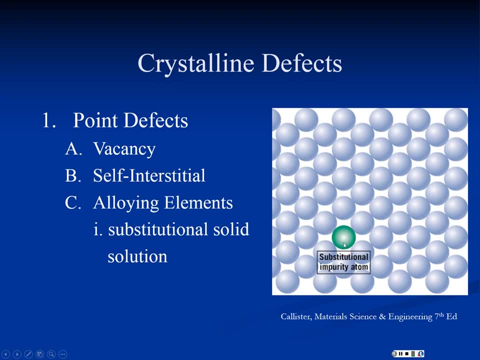 And there are four requirements for substitution. If you just think back, if somebody wanted to pretend to be you, what would they need to have? What characteristics? Well, they need to be about the same size as you. They'd have to look the same. 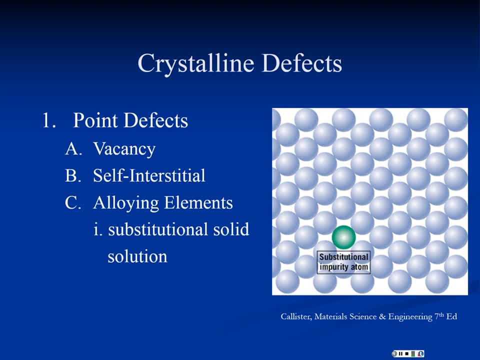 That's the exterior, would need to look the same Personality-wise. they need to be able to pass off as you. So if you're really energetic and social and they're a wallflower, they're not going to do a very good job of pretending to be you. 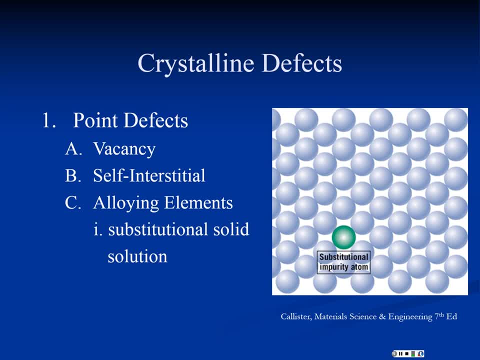 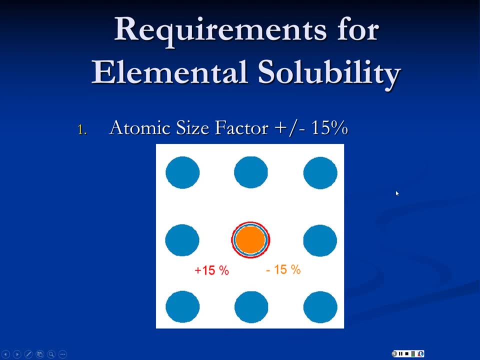 So you're going to look for those kinds of things. Similarly, the atom here has to play the role of the atom it's substituting for. So what do we need? Well, similar size, it needs to fit. It doesn't have to fit perfectly. 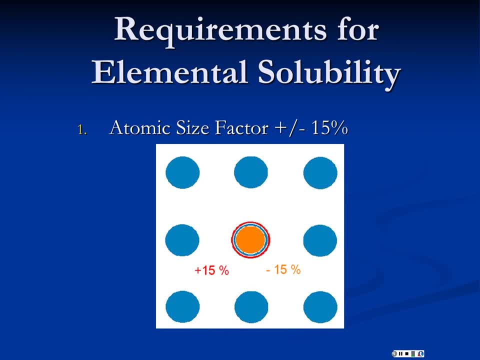 but if it's within about 15%, it can substitute very, very well. Now we're going to make alloys all the time with atoms that don't fit perfectly And that's going to create complications. It's not that we can't substitute them. 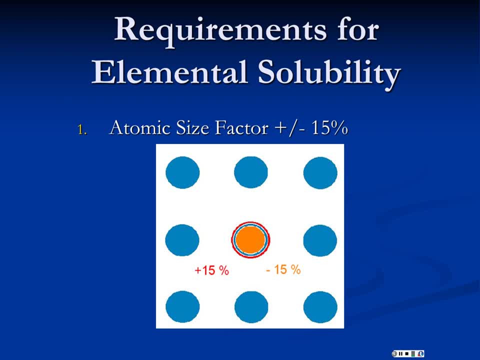 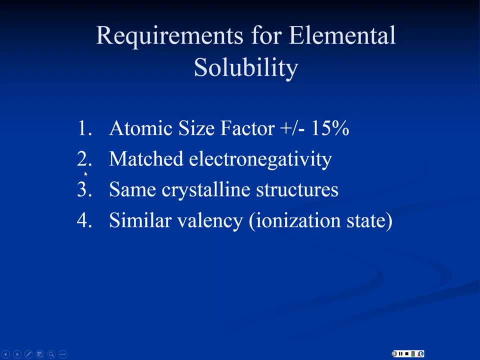 but there's going to be limits on how much we can do. But if you have good, if you're within 15%, you can substitute a tremendous number of atoms. The other three rules are that they kind of have to act the same. 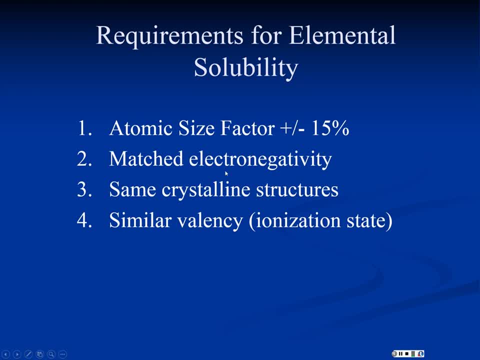 So they need to share electrons the same way They need the same electronegativity, So they have to participate in the bonding scheme the same way the atom would that they're replacing. They need to have the same preferred crystal structures. Why? 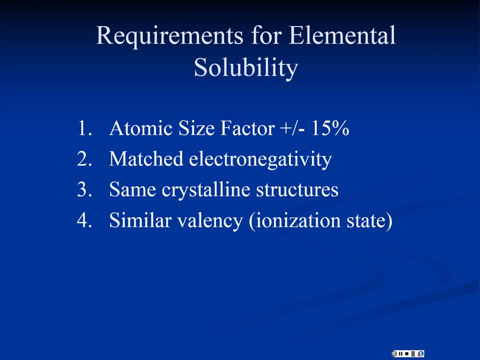 Because they need to want the same number of neighbors, or they don't. They interfere with the structure And then finally, they need to look the same. That is, the outside shell of electrons needs to be the same Similar valency. 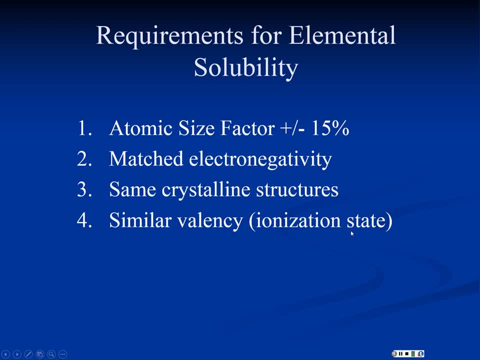 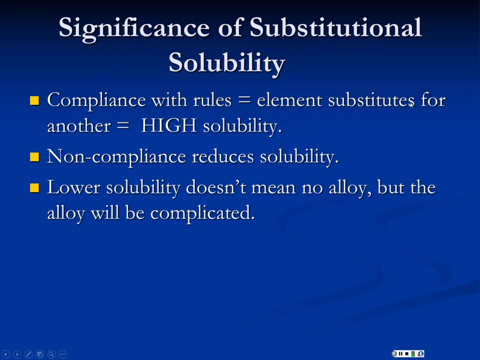 And if an atom satisfies all four of these, then you have tremendous solubility. Now why do we care? Well, if you comply with the rules, element substitutes for another, you're going to have high solubility. You can dissolve very large amounts of this substituting atom. 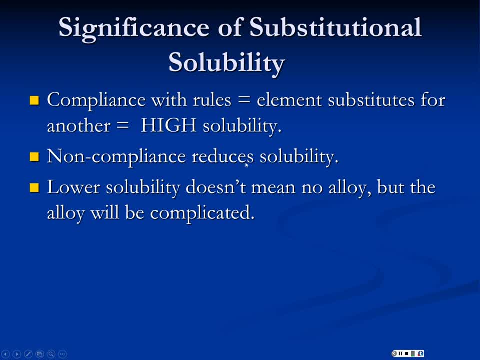 Non-compliance simply means lower solubility, And the worse your compliance is, the lower the level you're going to be able to dissolve will be Lower. solubility doesn't mean no alloy, but the alloy is going to be complicated. 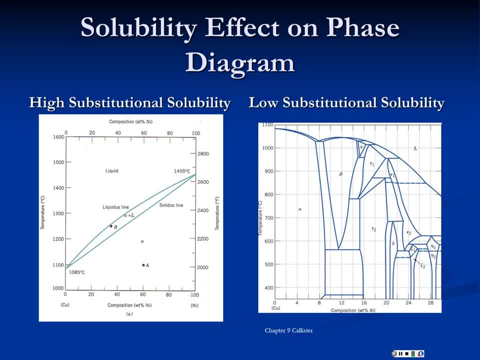 And I'll just give you a hint at what we're looking at. We're going to be learning about phase diagrams, And a phase diagram simply tells us what are the limits of solubility of one element and another. And in the left diagram we have copper and nickel. 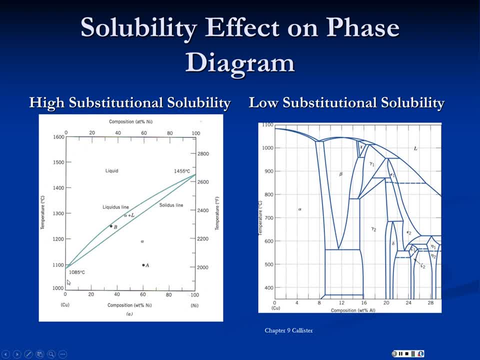 They are perfect substitutes for each other. And so what happens is we can start with pure copper, We can add nickel and add nickel and add nickel, And we never reach a point where you can't keep adding a nickel atom, Because there is no limit to the solubility of nickel and copper. 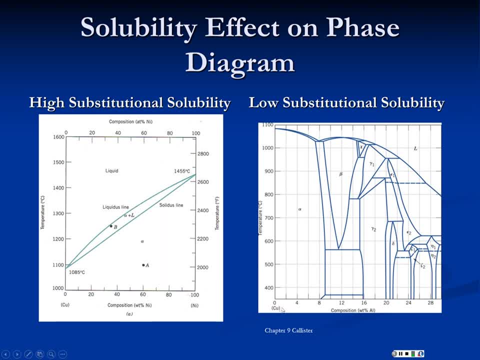 They're perfect substitutes. However, we can go to copper and aluminum And it turns out they're really bad substitutes. So we start with pure copper on this edge And as we add aluminum, we run into a vertical line. This line tells me that I can't dissolve any more aluminum. 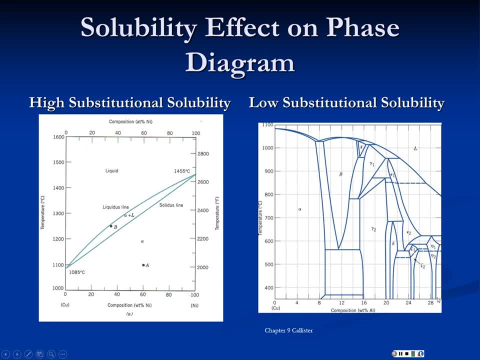 And you notice there's a bunch of vertical lines And we're only up to about 30% at this point. So we get a very complicated diagram as opposed to a very simple diagram. It's not that we can't make the alloys. 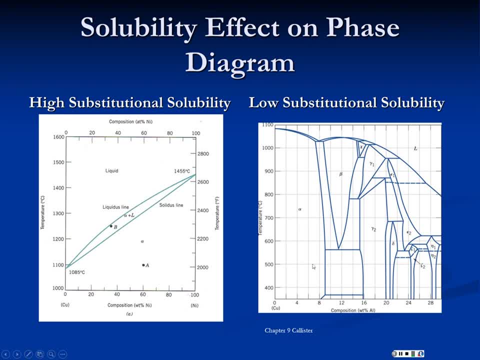 Aluminum and copper alloys are quite common, But they're very messy in terms of their structure Because this stuff won't dissolve. So we're going to come back, We're going to see these in a few weeks, But this is where solubility violations really show up. 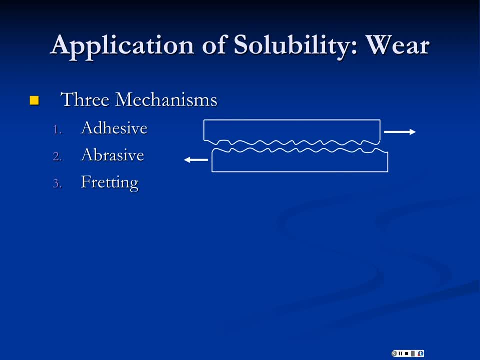 Another area we really care about solubility is in wear, And we will focus with some detail on all of these mechanisms in a few weeks. But the first mechanism of wear between sliding surfaces is called adhesive wear And the thing is, wear is one of the major causes of failure of all engineered components. 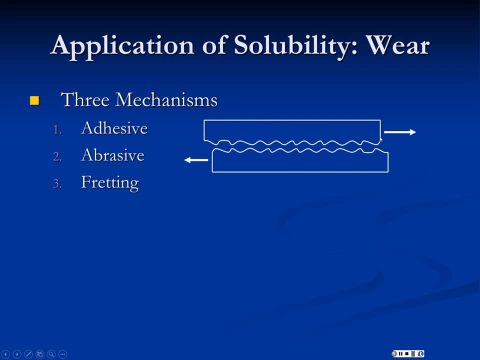 And it occurs when one surface slides past another. Now this is extremely magnified, It's schematic. But if you magnify any surface, it's not going to be smooth. These are called asperities. These are little bumps And the problem we have with rubbing surfaces or even rolling surfaces. 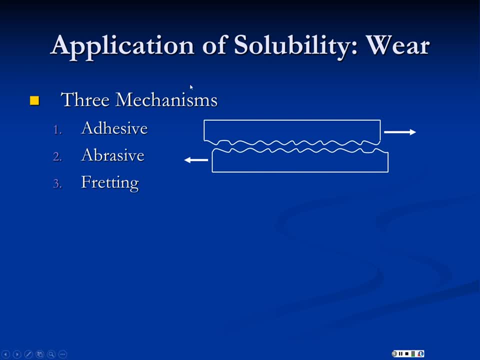 is that contact does not occur over the entire surface. It occurs where peaks meet And most of the surface isn't in contact. So the actual forces on those points are incredibly large. And what happens in adhesive wear is we have metals that are compatible. 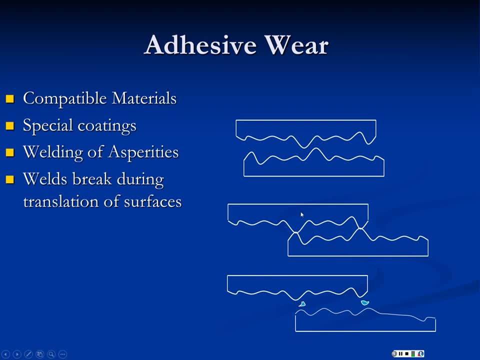 And when you do that, as things slide, you get contact at asperities, very high stresses, And if they're compatible metals, they actually will weld and fuse into a single piece. Now, as the sliding continues, you break those welds. 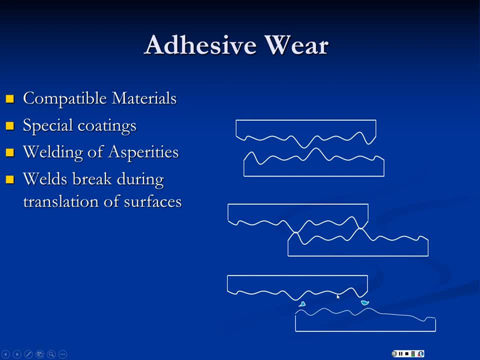 And in the process you break loose material And then other asperities touch and weld And so on. the process continues And you gradually break material loose from one or both surfaces Through this compatible welding process. Now, if we go to an engineering design book, 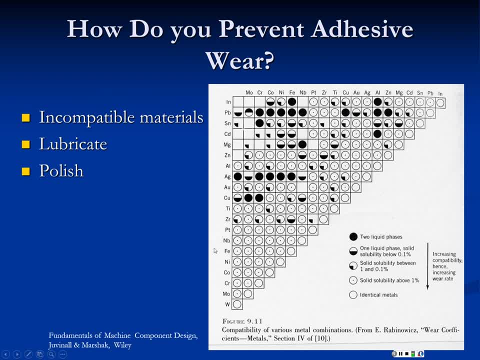 And this is the machine design text that we use for seniors in mechanical. You have charts like this And it basically tells you whether materials are compatible or safe to use together in a wearing environment where they're rubbing And you notice there are empty circles or circles with a dot. 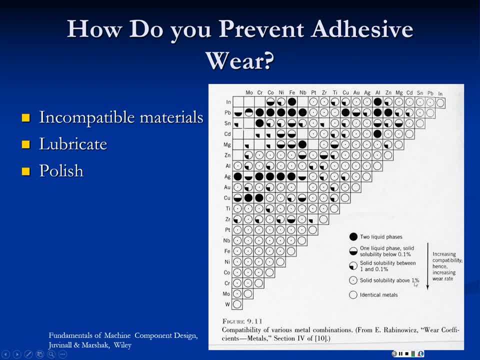 And that means the metals are ideal. They have very high solubility And you do not want to use them. They're too compatible. Now, as you fill in the circle, the pie charts, As you put in a little wedge here, 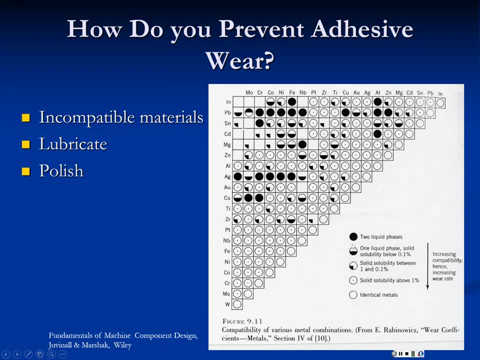 We see solid solubility is lower than 1%, But greater than a tenth of a percent. So they're still soluble, but not at a high level. So this is going to be a better combination. They're not going to suffer adhesive wear. 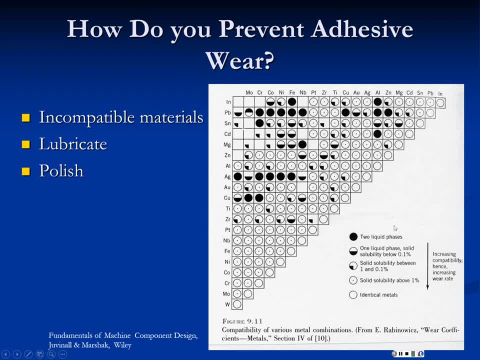 And the best materials, the solid black circles don't even have solubility in the liquid state, Let alone in the solid state, So they're completely incompatible metals And so you will not get adhesive wear. And this all springs from those four solubility questions. 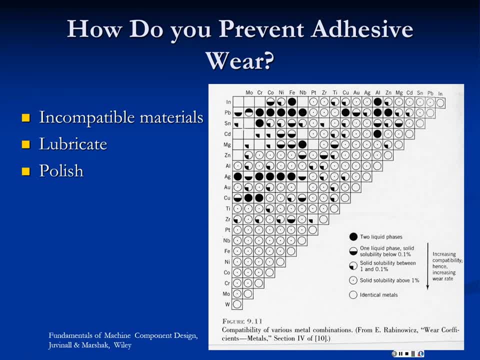 If you don't have a chart like this, you can ask those questions about the elements And identify then good, incompatible materials. You don't want them to be soluble if you're trying to prevent wear. So incompatible materials, We also will use lubrication that keeps the metal surfaces from touching. 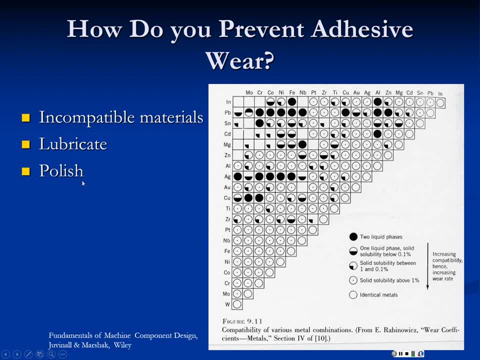 We'll also polish. Well, that reduces the height of the disparities. You get more contact, lower stress or lower force at each contact And less welding. Those are all techniques we may use, So we'll come back to this, But again, pause the video. 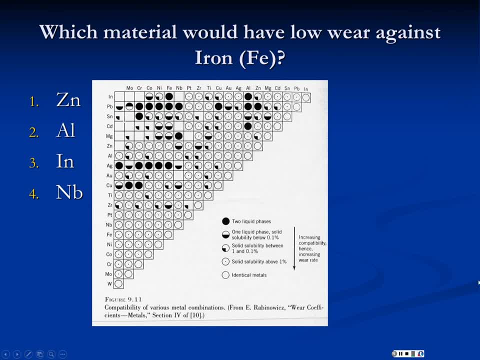 And can you identify which material would have low wear against iron? So you should have identified pretty quickly that indium is the compatible one As you come down the web line. obviously Indium is a black circle. That's some good stuff. 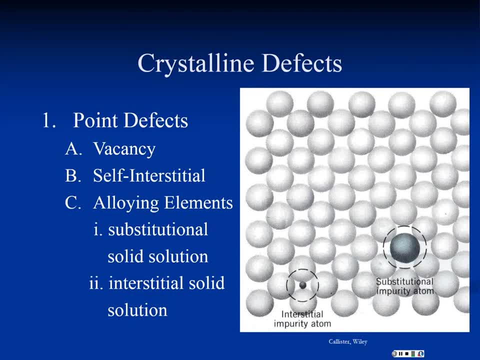 Okay, Continuing with point defects, we also have interstitial impurity atoms, And the key here is this atom is very small And will fit in between the lattice points of the parent element, And most of the time these interstitials in a metal will be nonmetals. 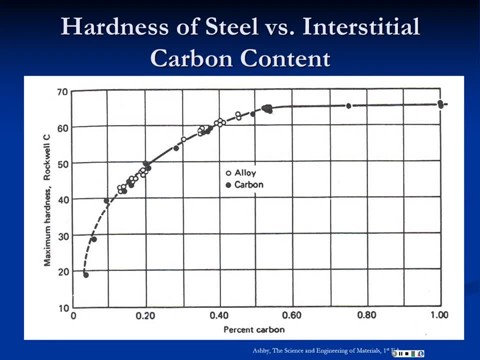 So what's the most important one? Well, we're going to spend a lot of time with steel- And steel is iron with interstitial carbon, And what we find is that as you increase the carbon content, the hardness of the steel rises very nicely, up to a maximum at about 0.55, 0.6%. 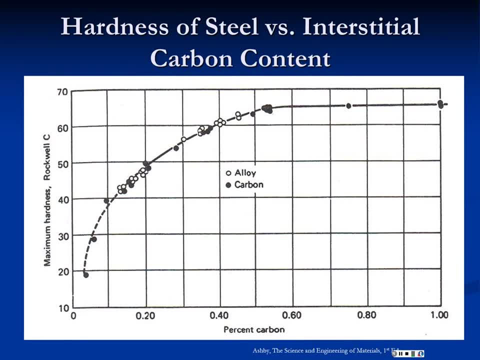 And of course then the question becomes: well, why doesn't it continue to rise after we reach 0.55 or 0.6?? Notice that it's pretty much flat. It levels out at about 65 Rockwell C. 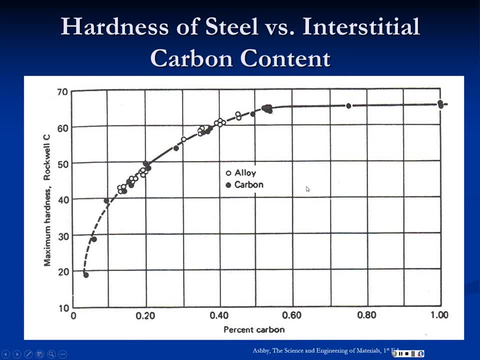 which you were using in the lab already. You've already used it in the lab, And that's about as hard as you can go with carbon-hardened or strengthened steel, And so we're going to have to wrestle with that, And we'll do that in a little bit. 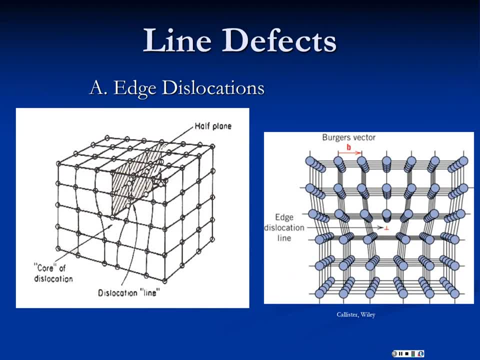 Okay, So that's point. defects for types. We also have line defects And there's a good deal of discussion in your text and in most materials science and materials physics books about dislocations. We're not going to get into the physics of how they move and doing all the geometry. 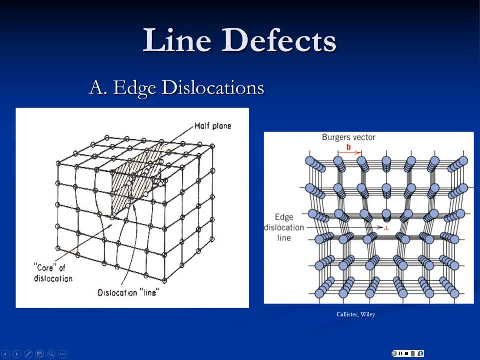 What I want you to understand is what they are and that they do certain special things. So this is an edge dislocation and it's simply an extra half-plane of atoms squeezed into the crystal. If you look from the end, then it looks like there's just a plane that's chopped off. 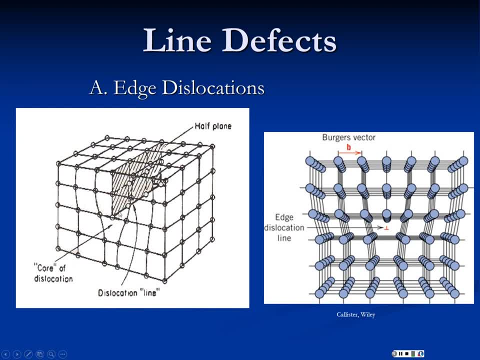 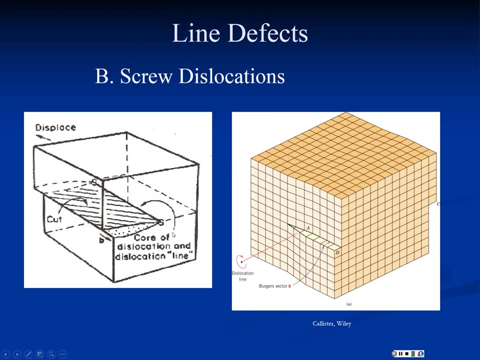 Now it doesn't necessarily go the length of the crystal. It may be only partway across a particular crystal cell or crystal grain, But it's an extra half-plane. Now, screw dislocations are a little more complicated, very difficult to visualize in their full three-dimensional state. 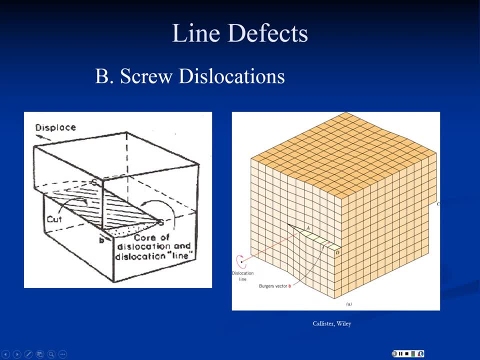 But think of taking a piece of foam and slicing it horizontally and then twisting the top half and reattaching all of the atomic bonds here and you end up with a little step. It's called a screw dislocation, because if you look down on it at the right angle, 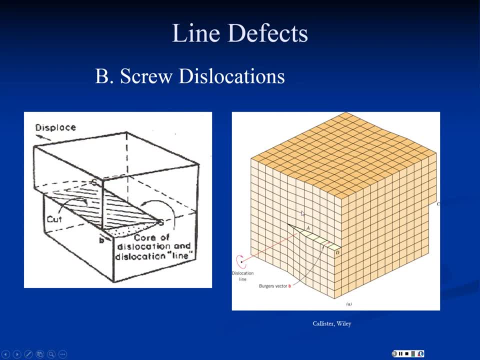 it looks like a staircase or a screw path that you've created. So, anyway, these are basically extra, partial, partial chunks of atoms, extra planes of atoms jammed in to the crystal structure. Now, why are they important? Well, and how do we know they exist? 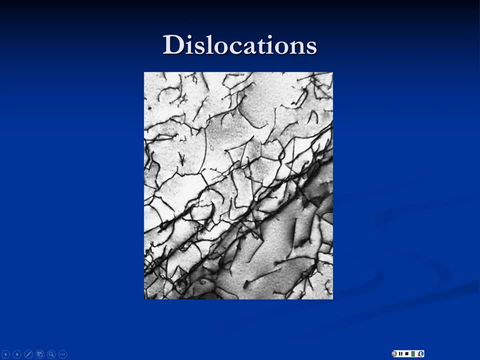 I guess we know they exist because we can see them. So these black lines are actually dislocations. This is transmission electron microscopy, And we're shooting a beam of electrons through a very thin piece of the material And what happens is where there are extra atoms packed in. 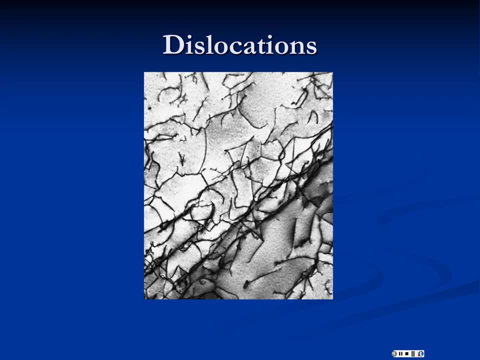 the beam is absorbed, It doesn't make its way through, And so we see light And the areas that are the minimum thickness, and then extra atoms start interfering with that light. So we're not seeing the atoms there, but these are essentially curtains of extra half planes of atoms packed in. 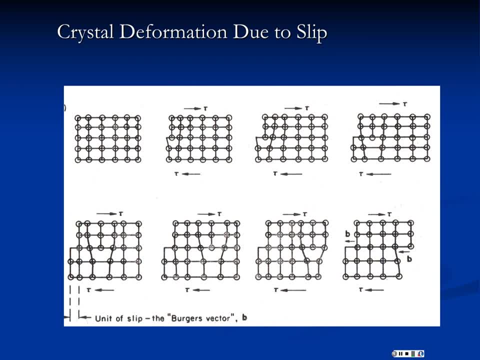 Now why do we care? We're going to deal with this in great detail in a few weeks when we talk about strengthening mechanisms. But we apply a force to a block of crystal material And so we're going to push it across to the right on the top. 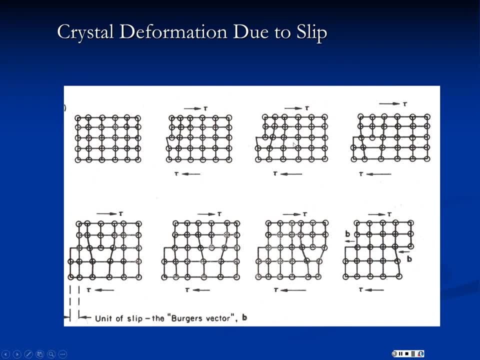 and to the left on the bottom, We can induce a dislocation. So a dislocation can be formed if this force is great enough, And so that's going to be one of the key properties we'll be looking at- And then, once we've made this dislocation, 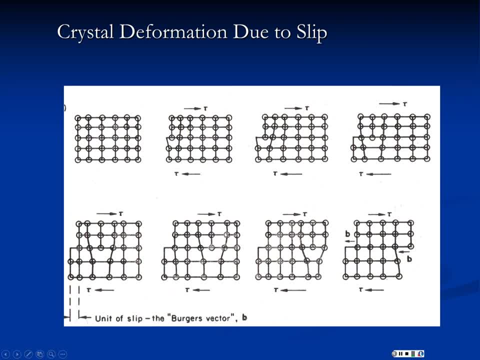 it's possible for this dislocation to just propagate through the crystal, pop out the other side and it looks to us now like we've slipped the top half of this crystal past the bottom half. but we've never broken more than one bond at a time. 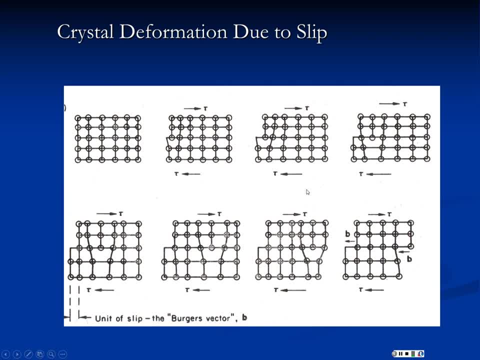 because of the way the dislocation works. So dislocations are going to be the key to most materials' ability to change shape permanently. It's how plastic or permanent deformation occurs. So you need to have this picture of them All right, And we find also that you know. 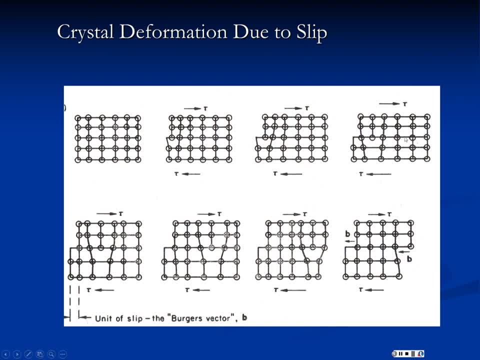 if you think back to what a dislocation is, there's a lot of energy involved. There's, these bonds are stretched. here These bonds are compressed. All of these atoms have elevated energy And if there's a dislocation here, it's going to be very difficult to form a dislocation. 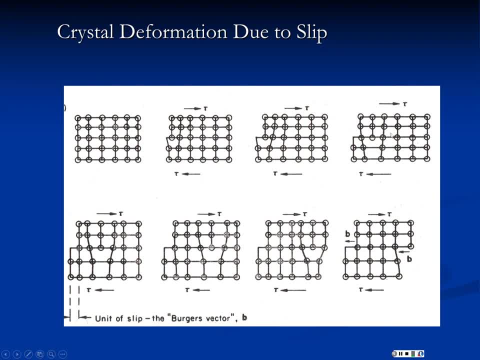 that's going to propagate or is going to exist in this region because of the elevated energy that already exists. So dislocations kind of exclude other dislocations. They get in each other's way because of the disruption they create. So one of the things we find is that the strength of a material 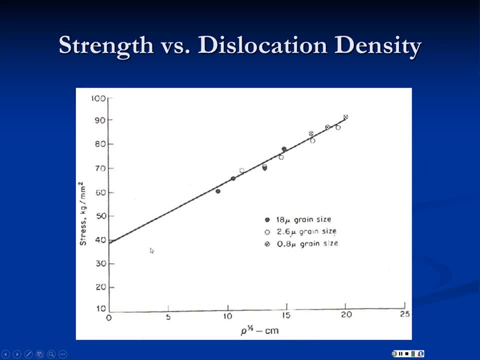 that is, the ability of a material to take in additional dislocations or the ability for you to move those dislocations around. the amount of force or stress required rises as I have more and more dislocations, So we're going to see how we make these. 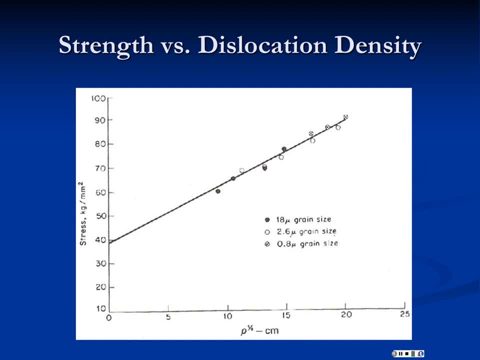 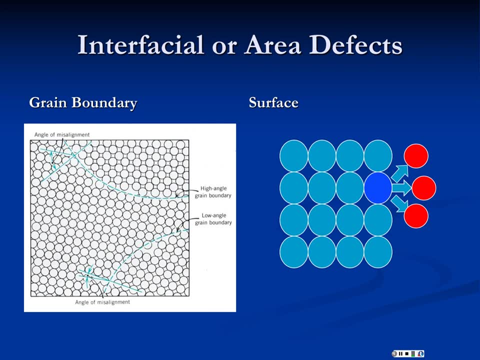 what they do. all of that's going to be very important. So, again, you need to understand what a dislocation is All right. And then we finally have area defects. So we started with point to line 2D, to area defects. 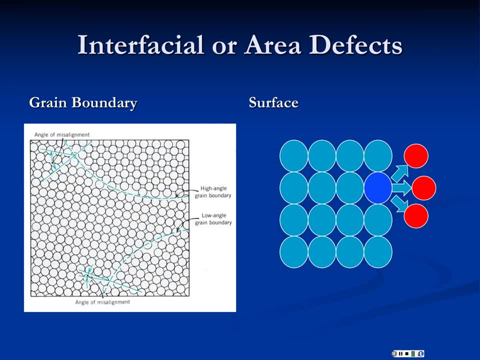 And area defects are. there's three types. The two that we're going to worry about the most are grain boundary and the surface, And we've already defined grains where they come from: from the solidification and the different orientations of the nuclei that form. 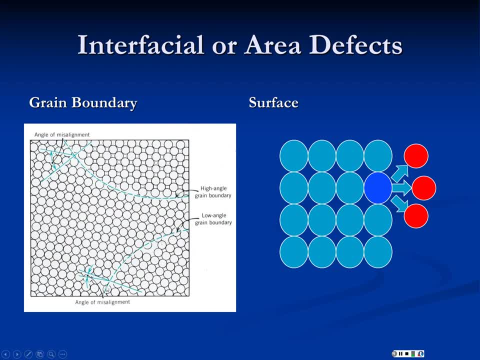 But where those grains meet, the atoms do not pack perfectly And in some cases they're pretty close to well packed. That is, if you draw a line through these atoms and draw a line through these atoms, they come together at a fairly low angle. 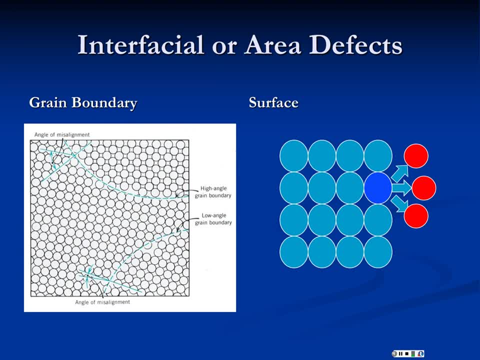 And so we call that a low angle grain boundary. That is, they're close to aligned, And so the energy of a low angle boundary is going to be low, because they're not that far from an ideal neighborhood. A high angle grain boundary, on the other hand, is a big mismatch. 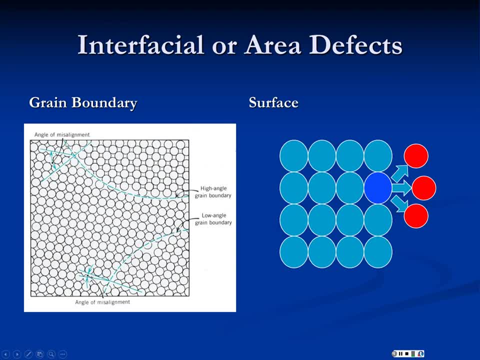 And so you're going to have a very high energy along this boundary, because the atoms are not aligning particularly well Now. a surface is an extreme version, because essentially what's happening here is it's not that you have bad packing, which is what the grain boundary gives you. 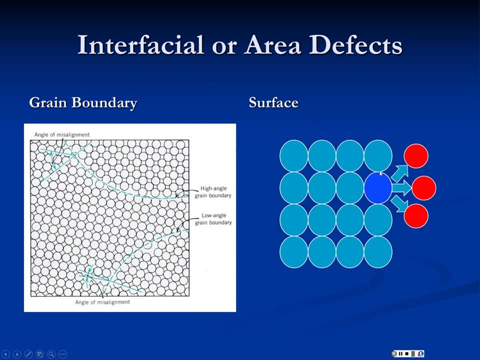 You just are missing all these neighbors out here, And so every atom on this surface- you're missing all of the neighbors to one side- is going to have very high energy, And in fact surface energies are often several times, maybe even orders of magnitude, higher than the energy of atoms in the interior. 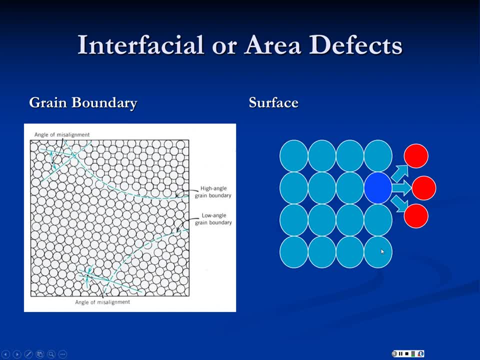 And it's this factor, this very high energy of these atoms that are missing their neighbors, that is behind much of our interest in nanotechnology, because nanoparticles, essentially, are entirely surface. They have very few atoms that are not on their surface and that means they're very energetic. 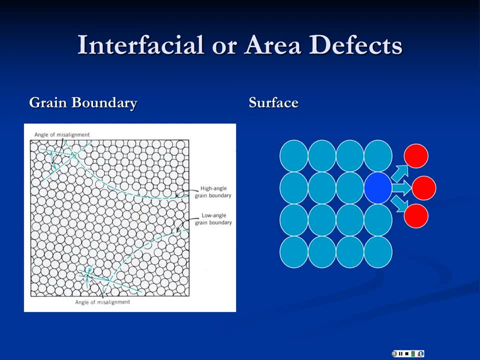 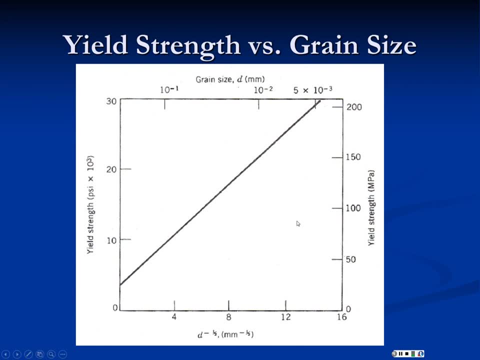 for the mass of the material that you're working with, All right, And so what you're doing in the lab is analyzing steel bolts and sectioning, looking at the microstructure and looking at the grain size, And so one of the things we find is that, as your grain size goes down, 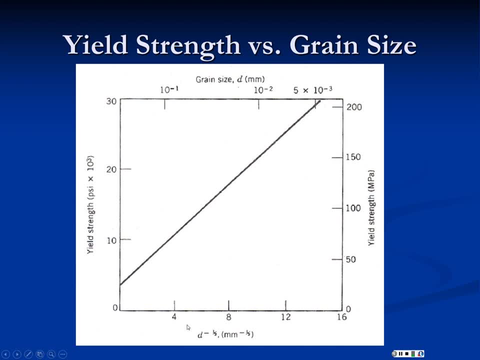 and so this is d to the negative 1 half. so as we go to the right this number is getting bigger. but d is actually getting smaller because we're dividing by the square root of the diameter, So yield strength or hardness. 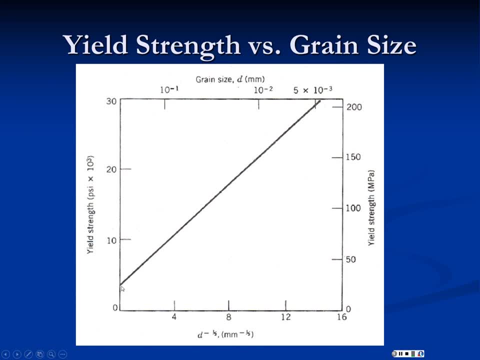 is maybe what you want to think in terms of Those are, as we've already said, essentially mean the same thing or imply the same effect. Your hardness is going to increase as the grain size gets smaller, And so there's the answer to one of the issues. 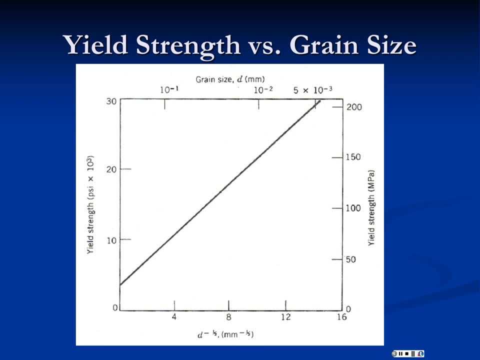 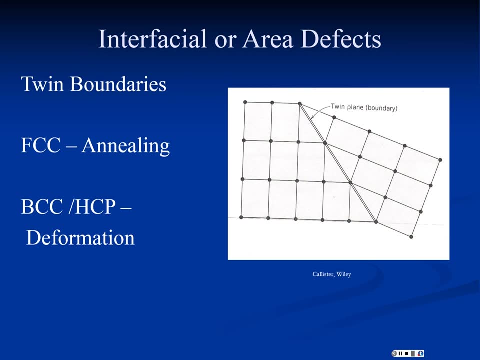 you need to address in your memos in the lab next week. All right, The last kind of interfacial area defect is um very unusual. It's called a twin, And a twin is not a disruption in the same sense as a dislocation. 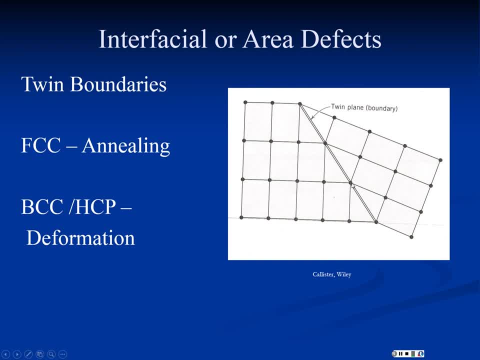 because, if you look, every atom on the twin boundary still has the same number of neighbors. So here's an atom in a perfect situation and he's got four neighbors. no big deal? Well, we still have four neighbors. but what's happened is you've folded along a plane. 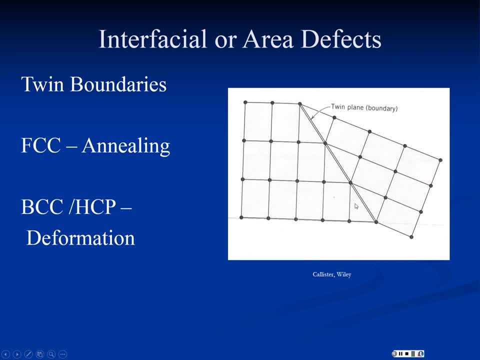 so the neighbor, the angles of these relationships are changed. So there's going to be energy associated with the twin boundary, because the angles are off But we're not breaking any bonds and we're not really compressing any bonds. So then, because we're not changing who the neighbors are, 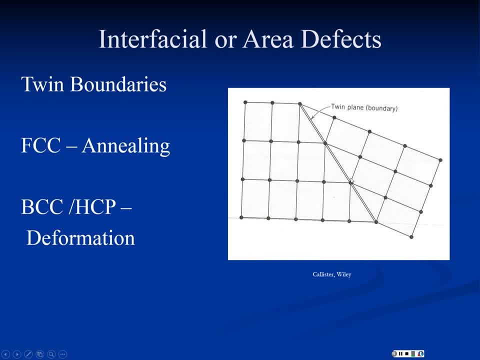 twins can occur in ionic materials, So you will see these in materials where these are alternating pluses and minuses, because if this is a plus and these all started out as minuses, well we're still surrounded by minuses. 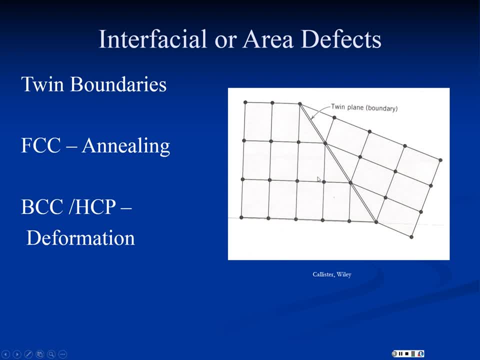 And we haven't shifted who the neighbors are, we've just shifted the relationship. In metals, twins are caused by different processes depending on the crystal structure. So in FCC materials, twins are usually caused by thermal history, by annealing of the material. 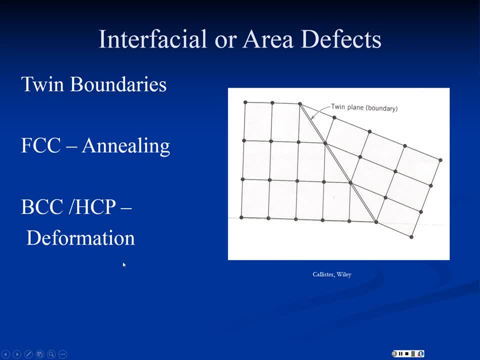 That's all that refers to is heating it up and cooling it down. In BCC and HCP metals, twins are a deformation product, So they're usually produced as a response to external forces which cause the part to deform. So you need to understand or remember. 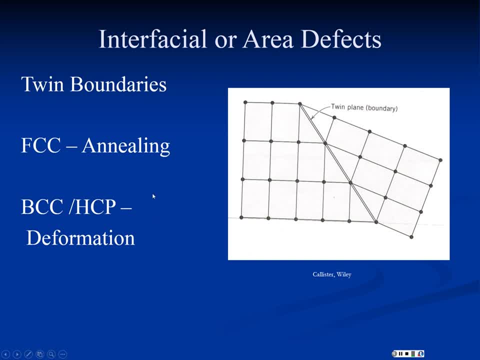 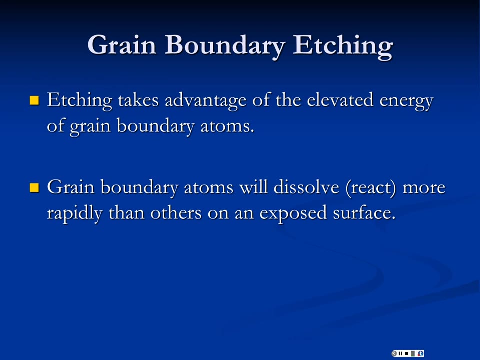 who gets which kind of twin, and we're going to look at a couple of applications that take advantage of deformation twins in BCC and HCP materials. All right, So all of these defects raise the energy of the atoms around the defect And the most significant to you in the laboratory right now. 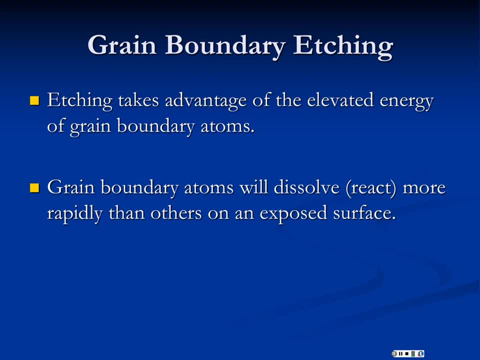 is the effect of the grain boundary on the energy of the atoms And what we're going to do. when you take that beautifully polished sample in the lab and you put acid on it after you cry, you're going to dissolve away atoms along the grain boundary. 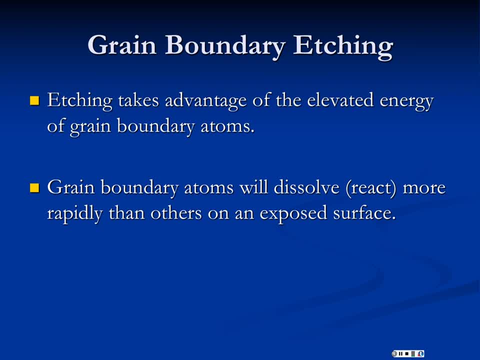 And the reason that's going to happen is that the atoms that are right on the grain boundary have the elevated energy of a surface atom because it's a surface you've polished, But because to their side is a grain boundary, they have extra energy from not having the right neighbors. 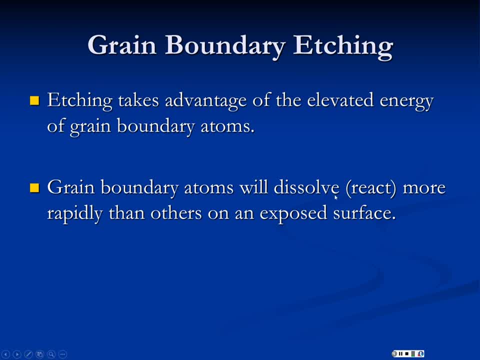 So they're going to be much more active, which means they will dissolve or react much more rapidly in the solvent And the acid. And as they dissolve away, you're going to actually dig a little ditch where the grain boundary is. The atoms are going to disappear. 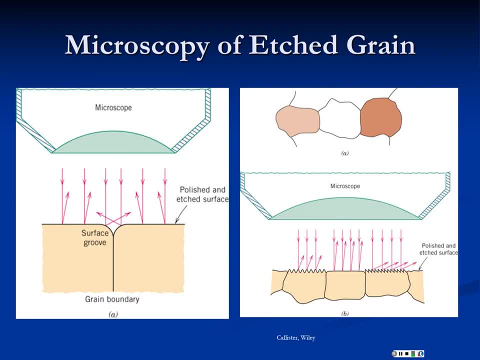 and you're going to have a hole there. So when we use a light microscope- looking at the left image here- your light microscope uses coaxial illumination. That is, you're like a Gould in Stargate: You have light coming out of your eyeballs. 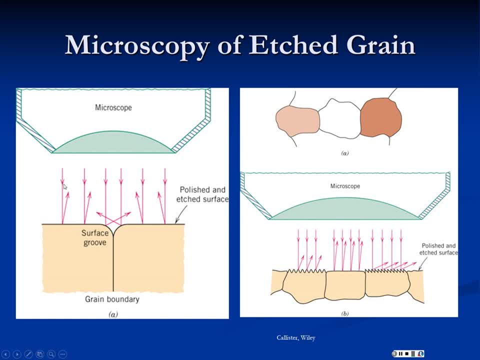 And as it reflects off the surface, it's going to bounce back and then your objective is going to send it over. You're going to see it So that illuminator you have built into the microscope means the light is coaxial with your vision path. 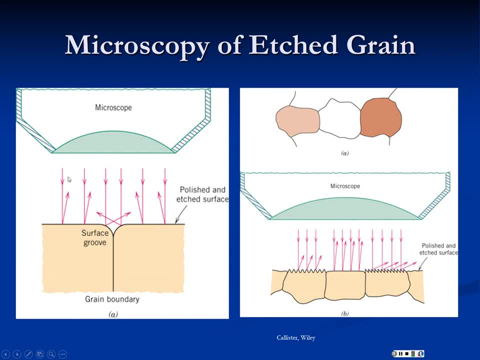 Where it's a smooth surface, that light comes back and you see it as white. Where we have a groove, now the surface is sloped and so light that strikes is going to be reflected to the side. It does not come back to your eyeball. 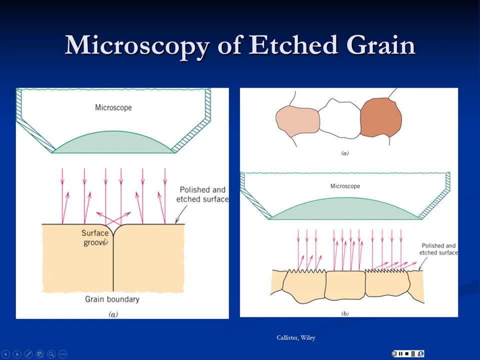 You just see this as dark, And that's how you see the grain boundary. Now it's even more complicated than that. There's even more information, because when we look, yeah, we'll get the grain boundary. so this is what you're going to see. 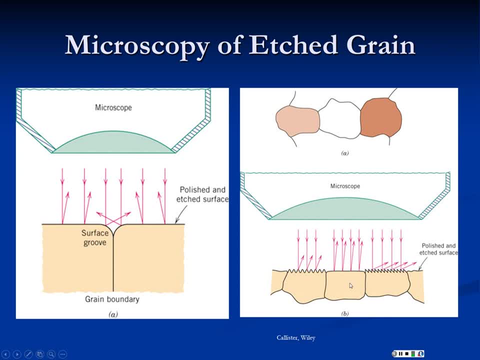 if we're looking at the surface. But different grains have different orientations, That is, they're sliced through the packed structure on different planes and that means the spacing of the atoms is different. The atoms on the surface right here are very close together. 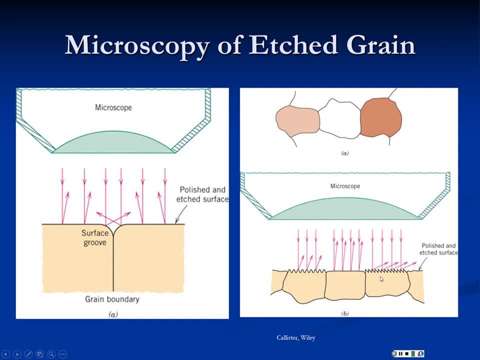 Here those atoms are spaced a little farther apart because of the way the crystal is cut, and here they're very, very far apart. All of these atoms are reactive, more reactive, So some of these will dissolve away. You're going to get little roughness to the surface. 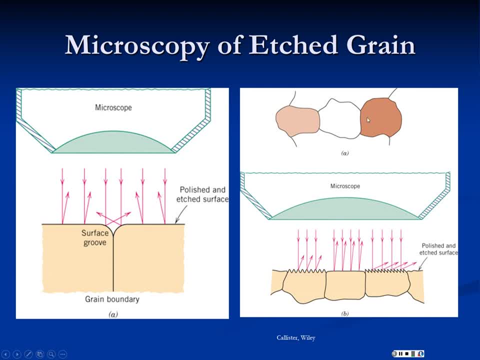 and so that scattering will make that grain look dark. This grain is almost perfectly smooth, so it's going to look very bright, and this one's somewhere in between and it'll look gray, So you get different intensities of the color. 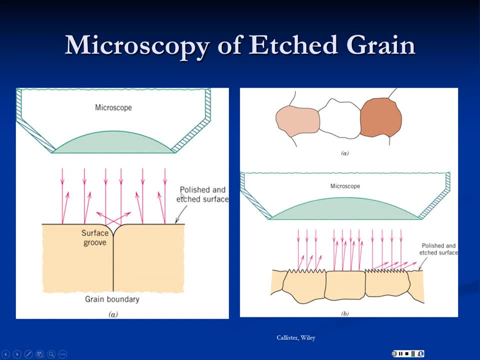 and it's not composition necessarily. It may be. You may have compositional variation in the grains, but most of the time it's simply because these were cut through different planes and the packing of the atoms is different and you're going to see different colors. 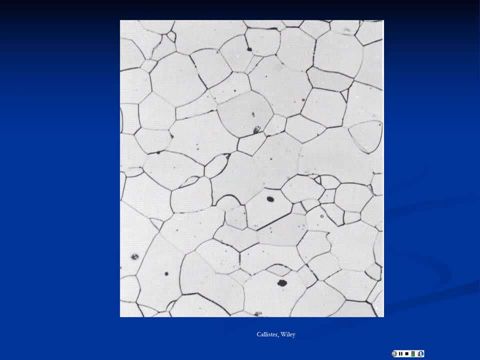 So let's look at some micrographs. Here is a classic image from Kallister. that's of brass and it's a fairly standard, pretty good polish. I don't see any scratches, But why don't you pause the video for a moment? 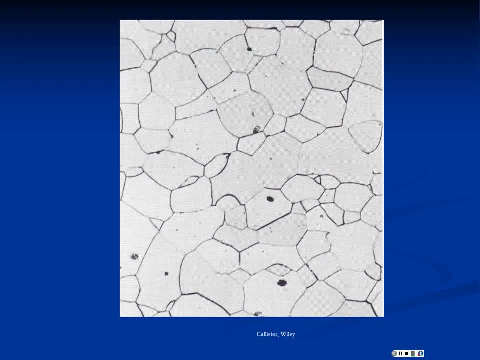 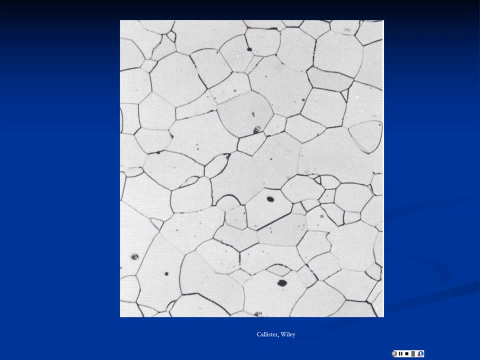 and see if you can make a list of observable features here and ask yourself: can you explain those features? All right, Hopefully you're back and you've got a nice list next to you. So, as you think about this image, you have just had a lot of theory explained. 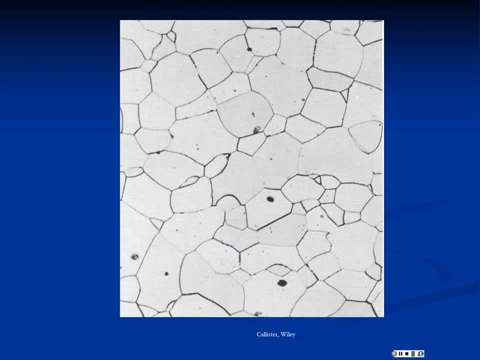 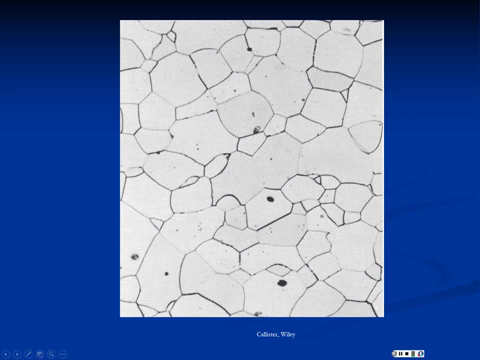 Energy level of grain boundaries. We've talked about solidification mechanics- last class, last discussion- And so you should be able to make sense of a lot of the features you're seeing in this image. The first thing you ought to notice is that all of the grain boundaries are not the same intensity. 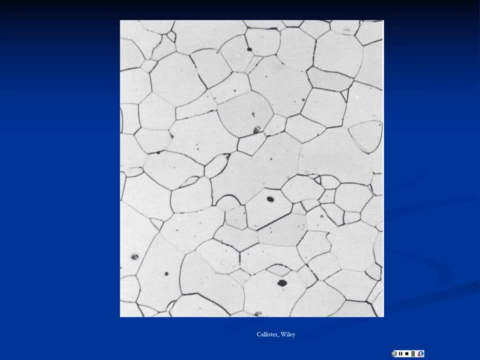 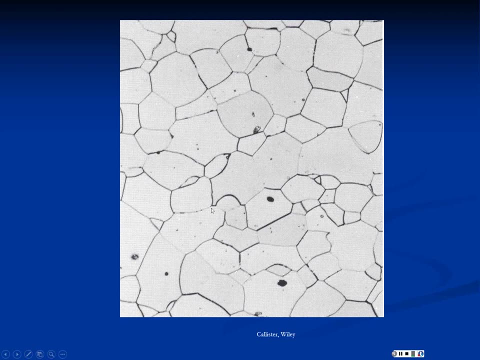 Some of them are dark, some of them are light, Some of them are curved, some of them are straight. Now, why would some grain boundaries be darker than others? Well, the ditches are obviously deeper, which means you have more atoms dissolving. 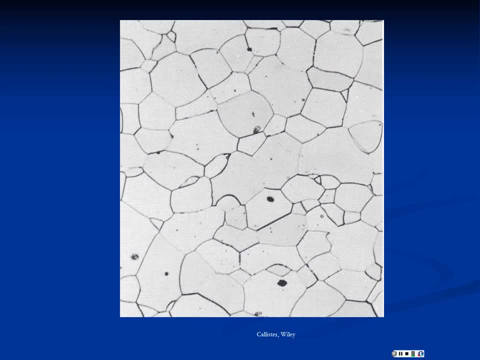 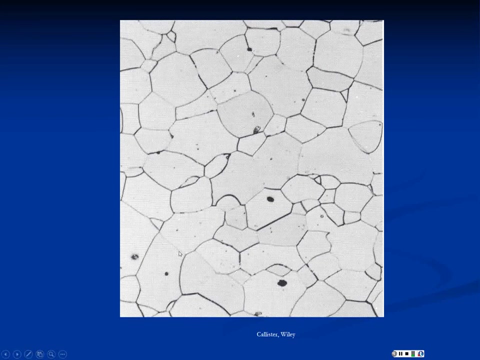 and more atoms dissolving means they were higher energy. Higher energy means it was a bigger mismatch. So the dark lines correspond to high energy grain boundaries. The light lines mean this one that you can barely see here implies that those grains almost were perfectly matched. 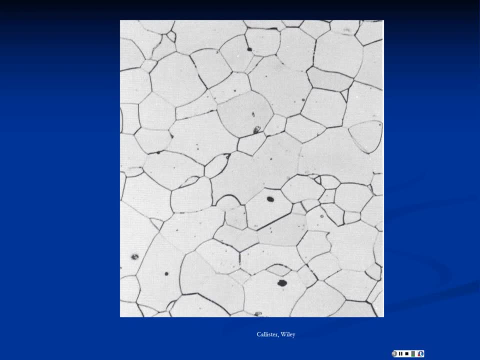 They're almost lined up, nearly a single grain, And in fact if you were to heat this for a long time in an oven, those grain boundaries might disappear completely as the crystals recrystallize into a single grain. Other thing that you might notice is that straight lines. 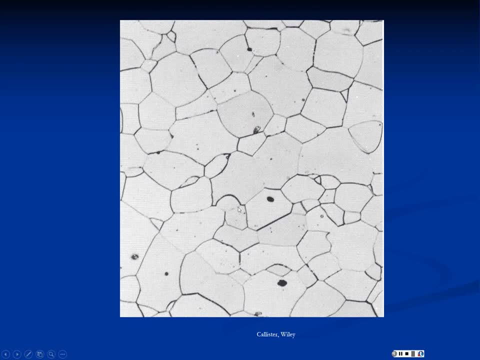 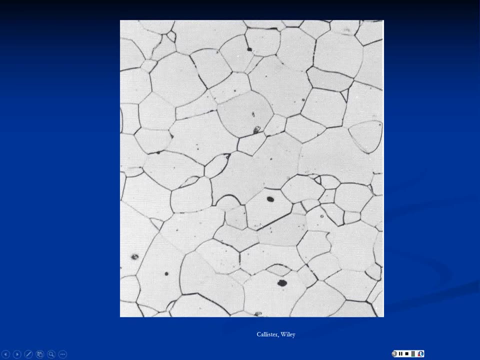 are very, very uniform. Curved lines vary in intensity, and so there's quite a bit of variation in the darkness along the curved boundaries, But straight boundaries seem to be very uniform. Well, the mismatch here is absolutely consistent. The two grains misalign. 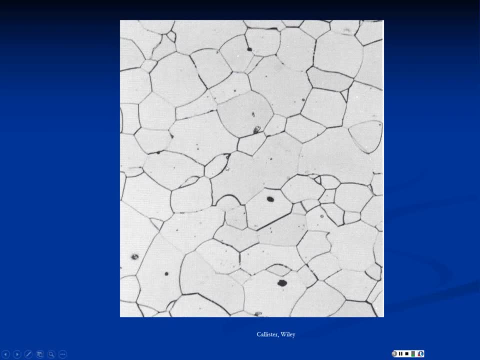 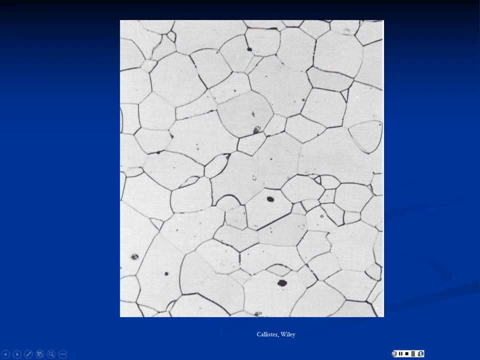 and you get the same energy level all the way. But as you come around a curve you're going to get varying amounts of mismatch, And so the intensity of curved boundaries tends to vary a great deal more than that of straight boundaries. You also see some little flecks in here. 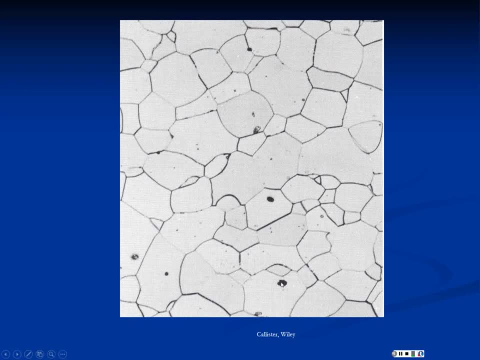 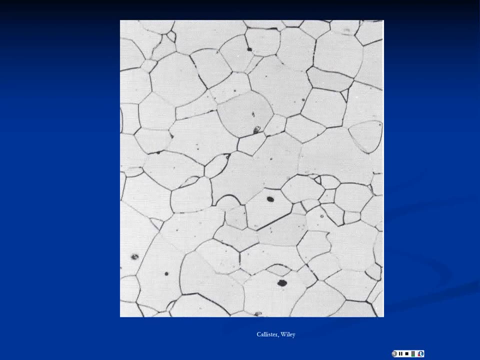 Little black spots, Little bitty ones and some big ones, And those are probably impurities or inclusions. An important lesson here is: there are no perfectly clean materials, And we're going to spend a lot of time discussing this as we get into failure. 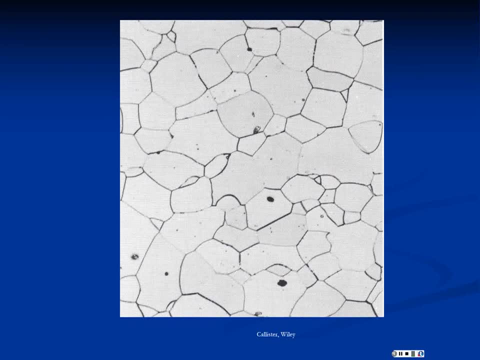 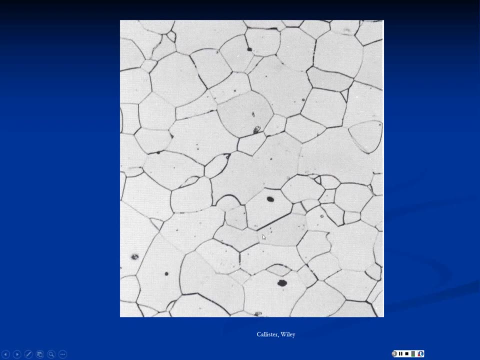 because one of your biggest problems as an engineer in specifying materials and in maintaining material quality is going to be controlling the levels of impurities, And a micrograph like this will give you a very quick sense of what your purity levels are. We'll do quantitative microscopy in quality control situations. 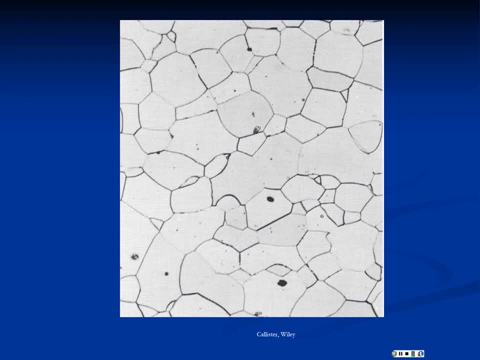 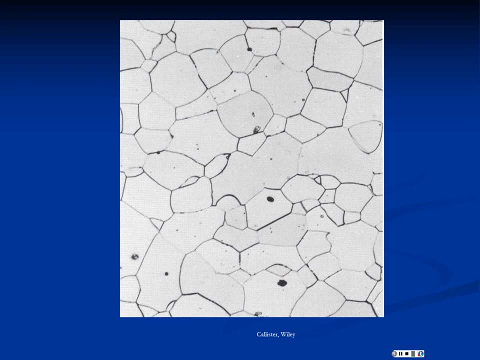 and actually use a computer attached to a digital image system to calculate what the percent of defects is, And we'll have bounds for that. So a lot of information here. This should make sense. It ought to look a little to you like a big mass of bubbles. 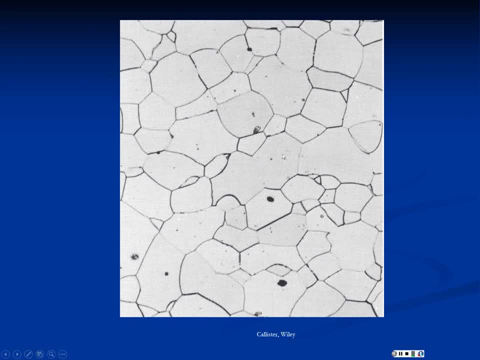 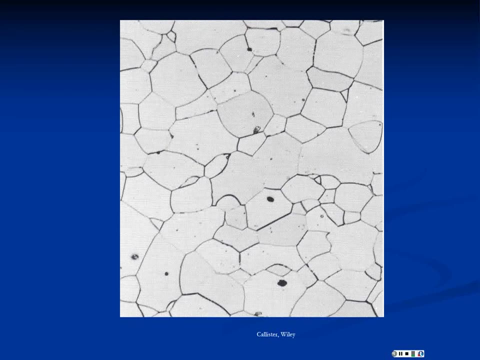 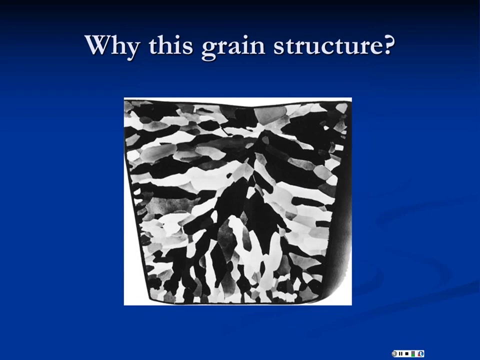 that have grown together. That's what happened, right, We were growing spheres of precipitating solid from the melt And those spheres run into each other and you get these truncated bubble appearance And it's a classic microstructure. Now, microstructures can vary a great deal. 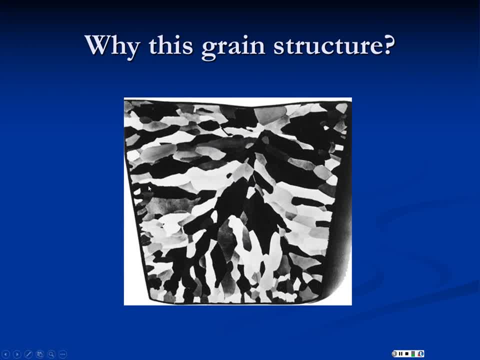 Here's a casting, and you see the grains are very, very long. And they're very long because solidification begins at the walls. The heat has to be removed through the walls, And so it's a lot easier for atoms to come over. 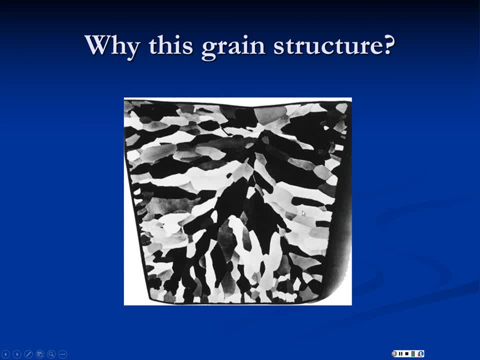 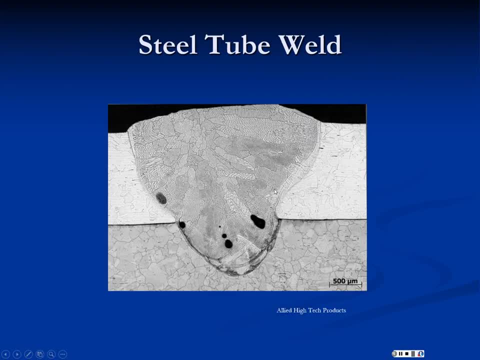 and give up their heat and join an existing crystal than it is to form another one. So you'll tend to get these long grains in a solidification process Weld. This is a weld in steel tubing. So here's the two pieces of metal that are being fused. 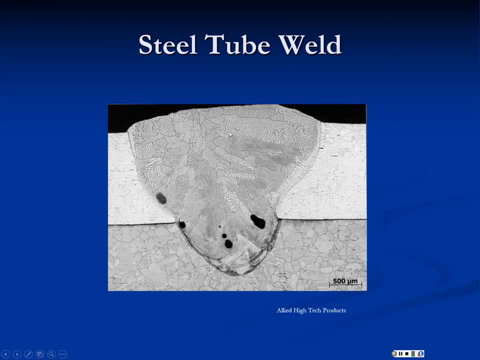 And obviously in welding you're melting and then recasting the material, And so again, long grains, because this was a molten pool. It is solidifying from the edges because the heat is being conducted out into these two parts and you get a similar structure. 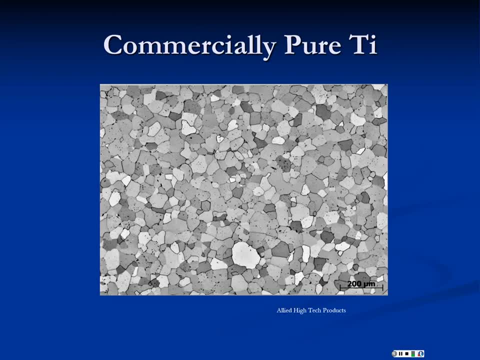 Now here's commercially pure titanium, And this is 99 point. I think it's two nines or three nines pure titanium, And what you see is there's no composition difference. These are all basically pure titanium grains, but there's a lot of color differences. 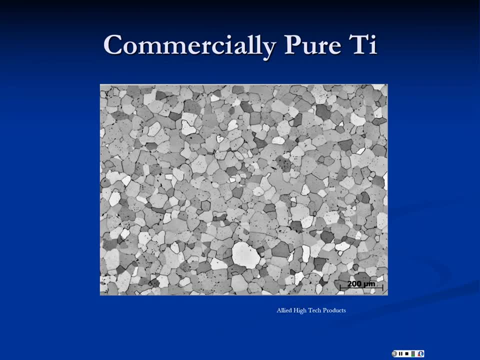 And those color differences simply have to do with the orientation of the plane, the surface plane that's cutting through that given grain, And so these dark grains. the atoms are probably pretty widely spaced, And here the atoms are as close together as possible. 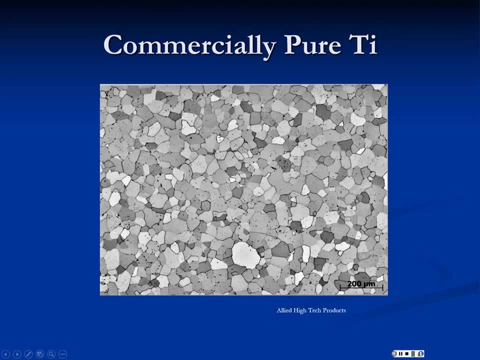 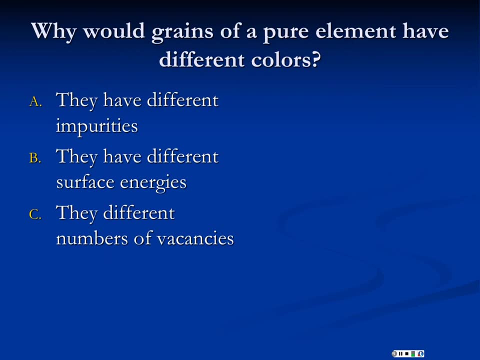 And so we get some dissolving of the surface and it produces a dark surface that scatters the light. All right, So again, why would grains of a pure element have different colors? We just told you You should know, Primarily they have different surface energies. 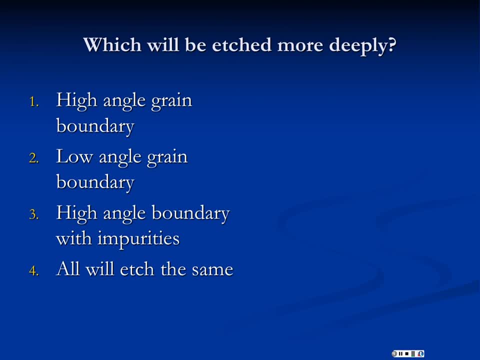 which is going to be etched more deeply- You may pause this and sort out the answer- And it should be a high-angle grain boundary with impurities. Why? Because impurities interfere with the bonds and raise the energy of the neighboring atoms. 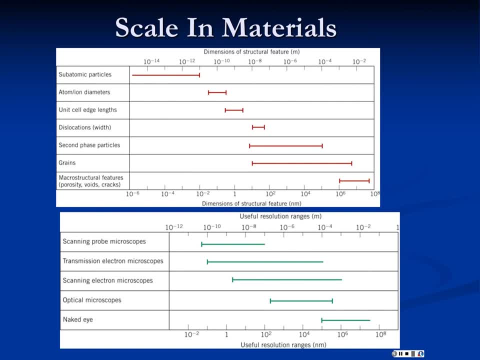 And we'll finish with this and I'm not going to spend a lot of time talking about it, but you need one of the challenges for students as we talk about defects microscopy and the next discussion we will be covering analytical techniques, electron microscopy and so on. 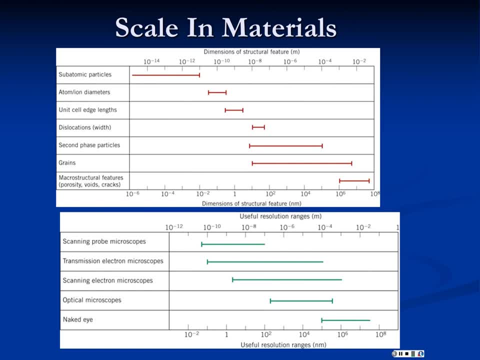 is identifying the tool for the problem. What is it you need to see? And so what tool are you going to go try to use, And the key is having some sense of the relative scale. So these graphics are from your texts and you need to spend a little time playing with them. 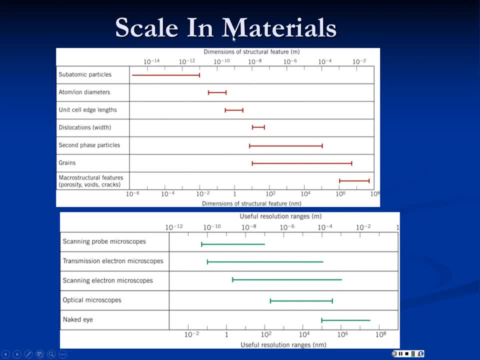 understand the relative scales And this is really nicely done because it's in terms of meters and because we're engineers, we really like to think in terms of 10 to the minus 3,, 10 to the minus 6,, 10 to the minus 9,, 10 to the minus 12.. 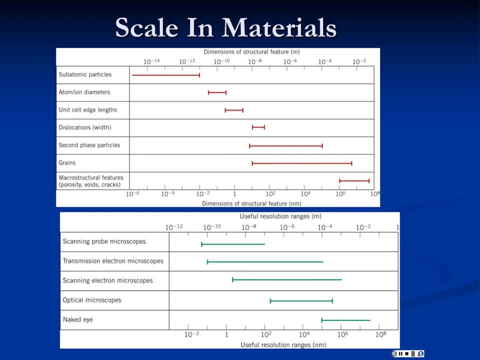 And if you really just kind of have some idea of what's useful at those ranges, you'll be well equipped to deal with things. So we're going to talk about this next class as we develop. how do electron microscopes work, how they differ from optical microscopes.